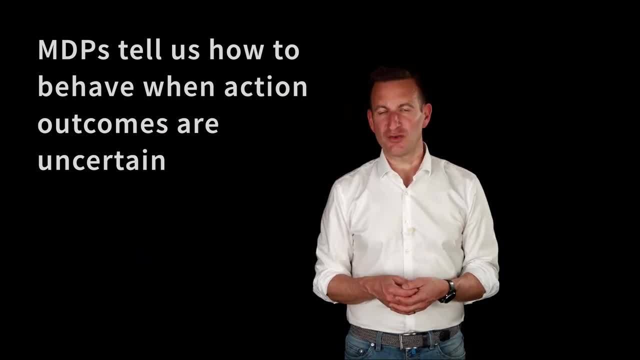 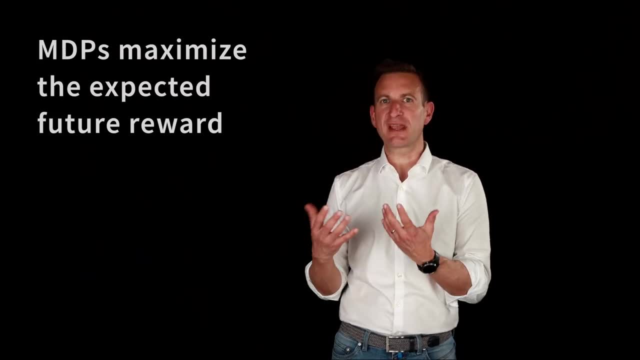 is some random component to it, then the MDPs allows you to make optimal decisions. What the MDP does? it maximizes some expected future rewards. So whatever you will gain in the future will be taken into account in your decision making process And the MDP can be defined with. 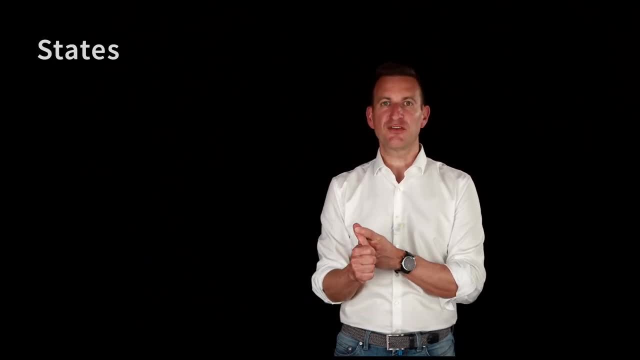 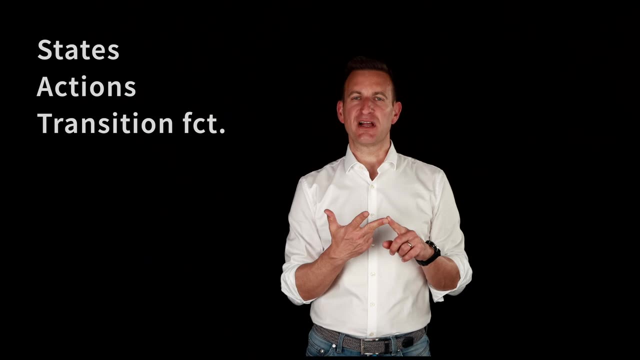 a four tuple. So you need to define what are the possible states your system can be in, what are the possible actions that you need to execute. Then you need to specify a so-called transition function which tells you: given I'm in a certain state, I'm going to execute an action to reach. 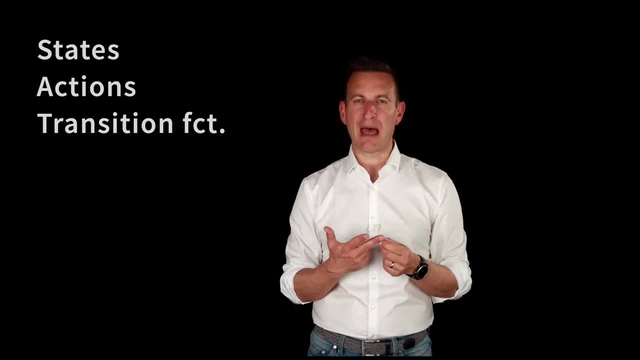 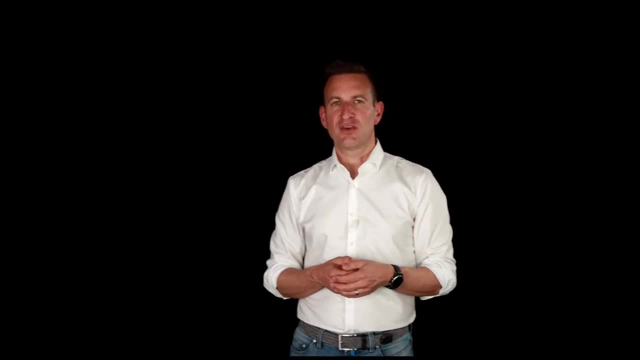 another state? What's the probability of this going to happen? And last, it's classifies the reward. What do I gain if I'm in a certain state? What's a good state? What's a bad state? So you can make a very simple example. For example, we have a mobile robot that lives in a 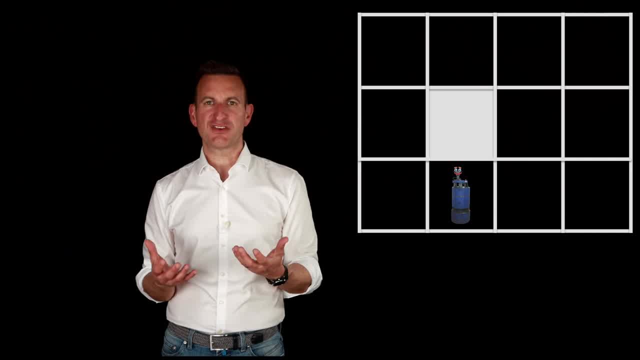 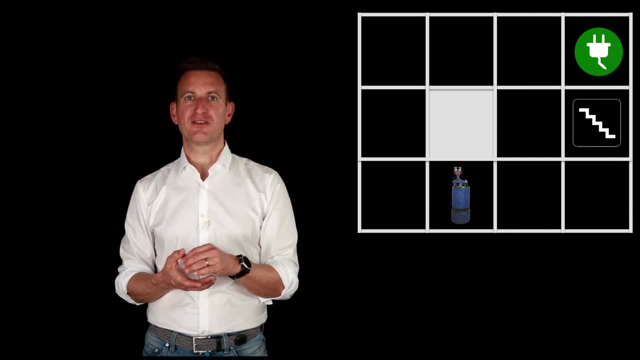 very simple world And there is one state where a charging station is where the robot gets its energy, so a positive reward. Or there's a staircase where the robot may fall down the staircase, so a place we want the robot to go. So the robot is somewhere and wants to reach the charging. 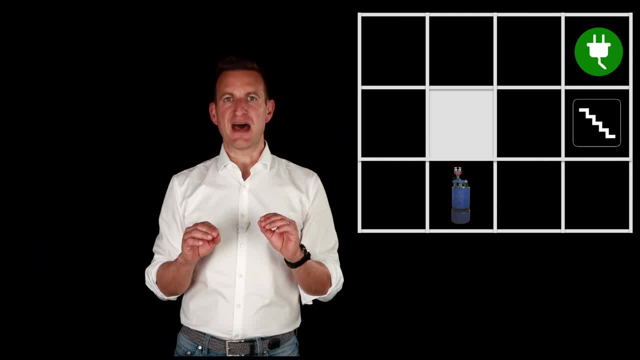 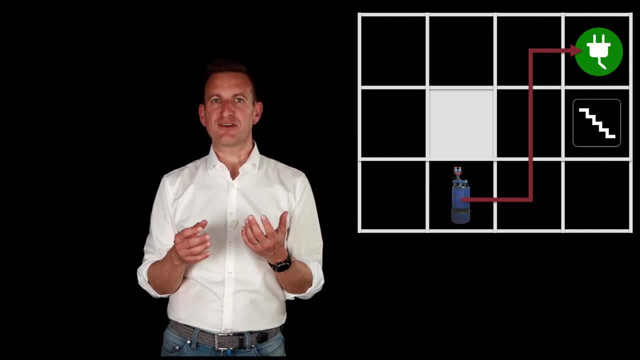 station. What should it do If it would perfectly know what it does? so perfect action, execution. we would probably navigate along the shortest path to the charging station. If we, however, take into account that some unexpected thing may happen, the robot executes a random command in a certain 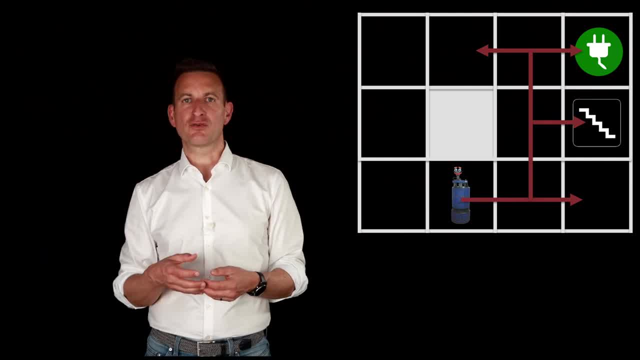 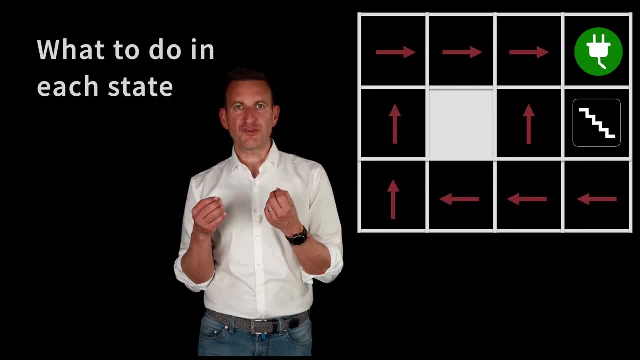 probability or a certain set of cases, then it can happen that the robot accidentally falls down the staircase. And how should we behave in order to avoid that? And what the MDP does? it tells you what to do in every state: a computer so-called policy which minimizes the probability of the 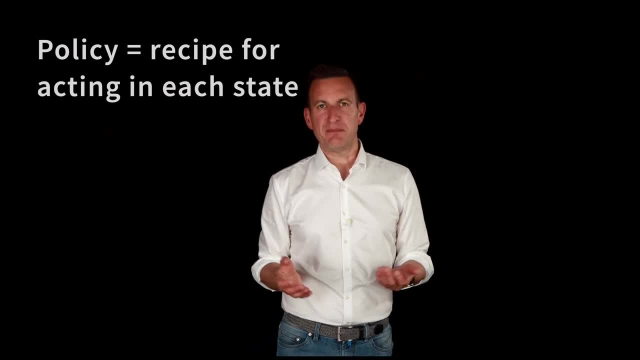 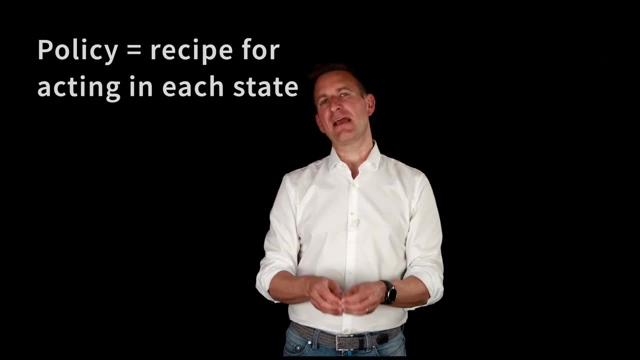 robot falling down the staircase. So the solution to an MDP is a so-called policy. it's basically a recipe which tells you if you're in a certain state, execute that action and this will maximize your expected future reward. And there are basically two techniques or two algorithms. 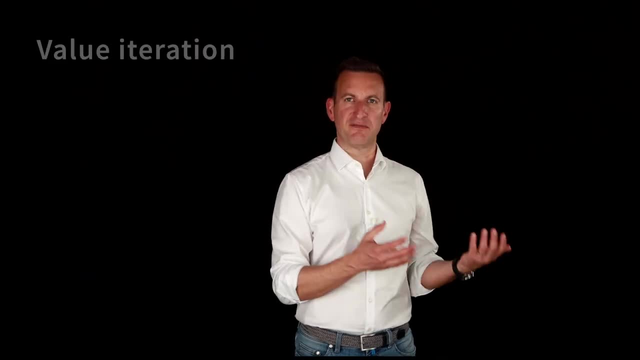 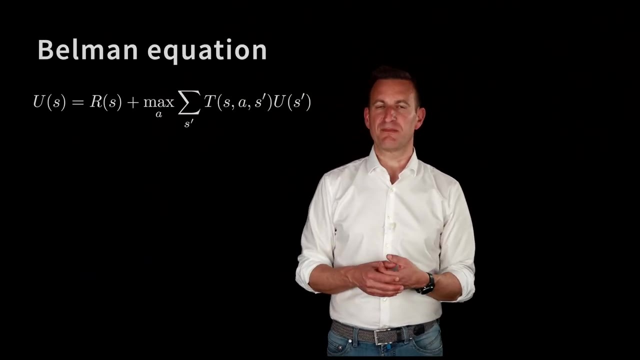 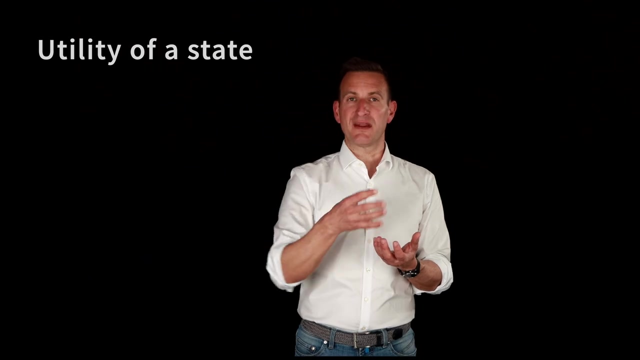 which allow you to compute a solution to an MDP. The first thing is value iteration, an approach going back to Bellman 1957, which optimizes the very famous Bellman equation And it uses a utility of a state and you can see the utility in what's the potential future reward that I can get, and that's